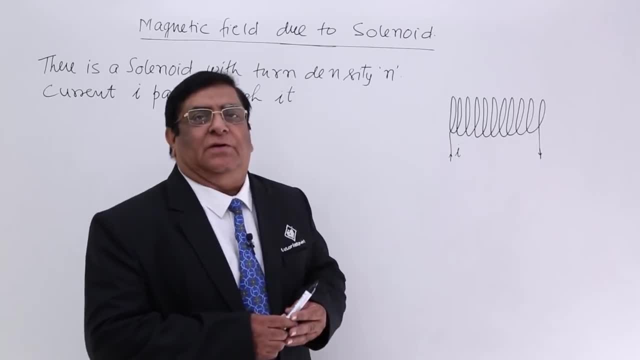 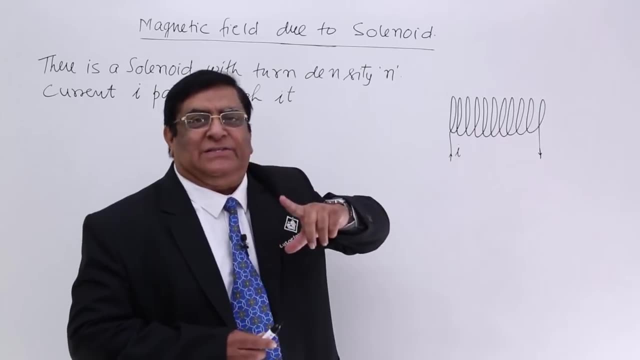 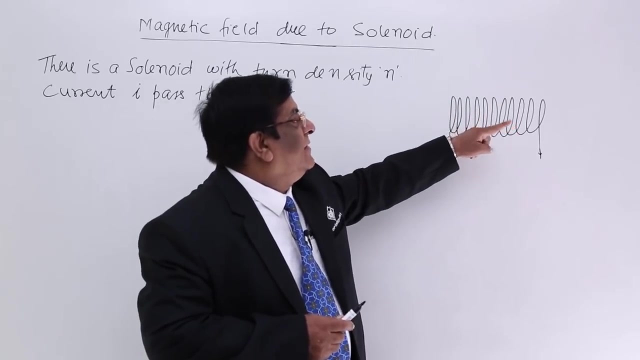 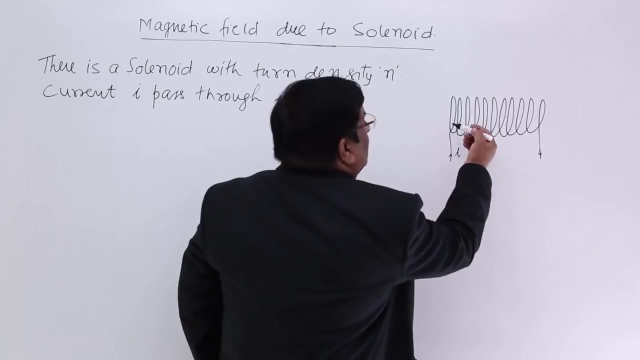 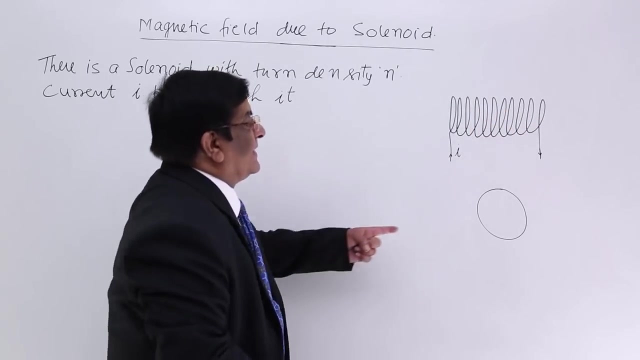 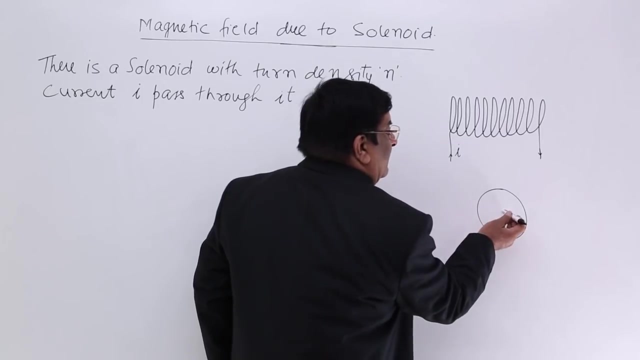 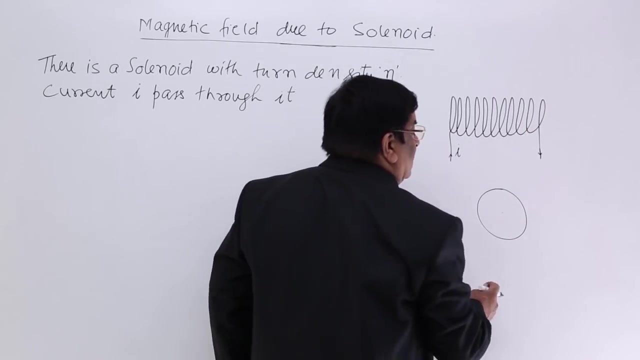 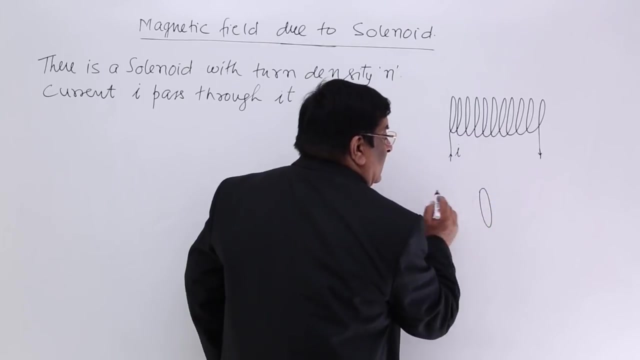 Now we are doing the most important derivation in Ampere's law, that is finding magnetic field inside a solenoid. What is a solenoid? Solenoid is a spring type. The conductor is made a spring. The coils, the different turns are not touching each other and the current pass through them. So any one turn is a circle like this. Then second circle, third circle, fourth circle and the current has to pass through all of them. Now if the current is passing through a circle, there will be a magnetic field at the centre of the circle and we have studied that this magnetic field is in this direction and when it comes out, it will go in this direction. That means, I will make it like this. If we have a circle this way, from here the magnetic field will come out and then it will go like this. This is magnetic field. After passing through certain distance, it will turn and come here to complete the loop. But what do we do? We make a second circle here. 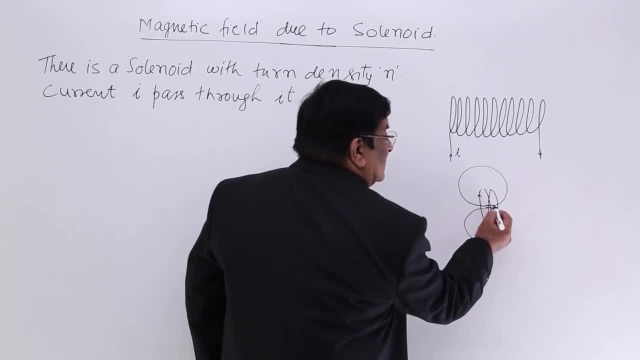 If we make a second circle here, at the centre, again magnetic field becomes straight and then it will go like this. But if we join a third circle, again it goes straight because at the centre, it has to be straight. So it is straight here and then it makes a circle. 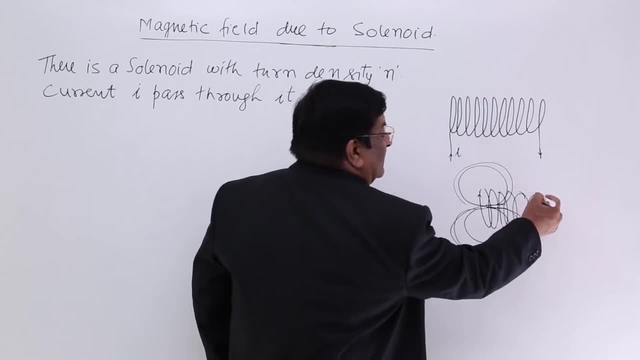 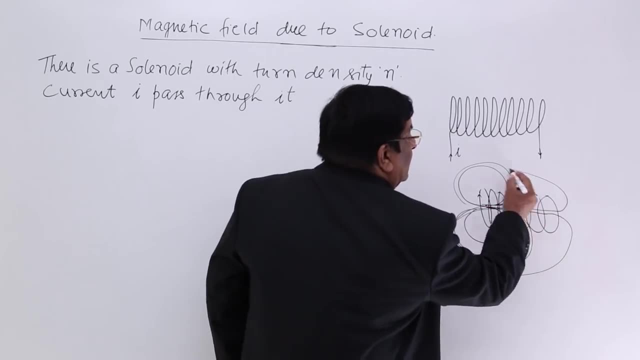 Now we join fourth, fifth, sixth, seventh circle and then it will go like this. If we make a third circle, it goes straight, straight, straight, straight and finally like this. 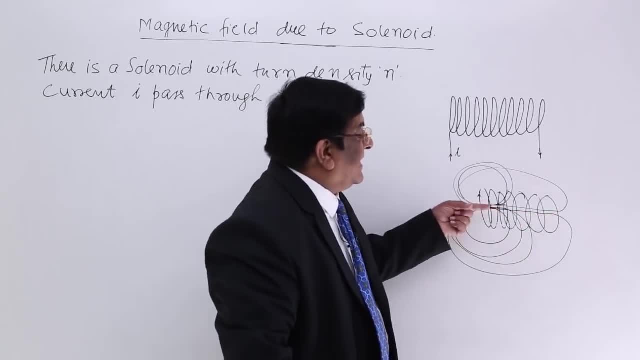 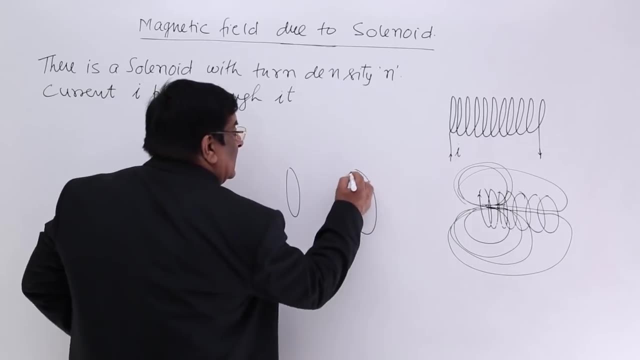 So what is the shape of magnetic field along the axis? Answer, it is straight. Again, if there are two circles like this far away, then from here magnetic field will go like this, from here it will go like this and here it is like this. This is magnetic field. 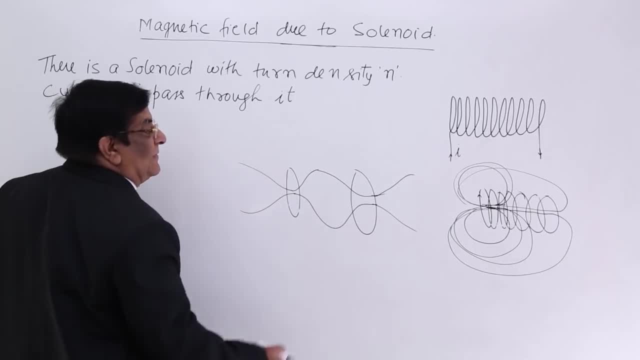 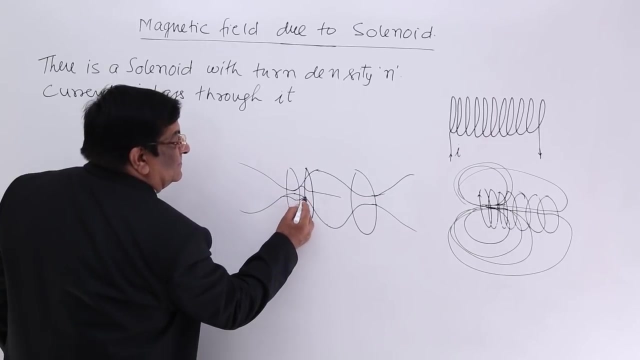 Okay? This way. But if you bring them closer, then this does not have space to reach this much distance. I put the current carrying coil here, then it will go here and become straight. If I bring it very close to it, then before it can increase its distance, before it will diverge, it has to go straight. 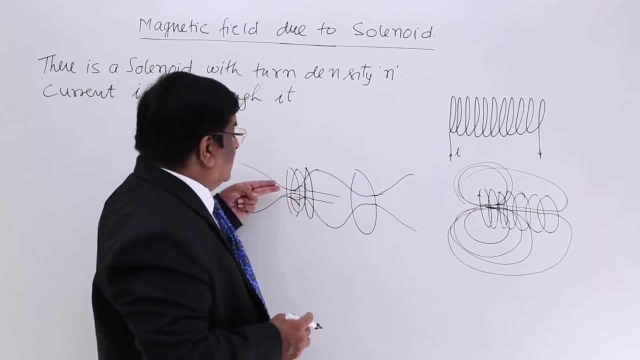 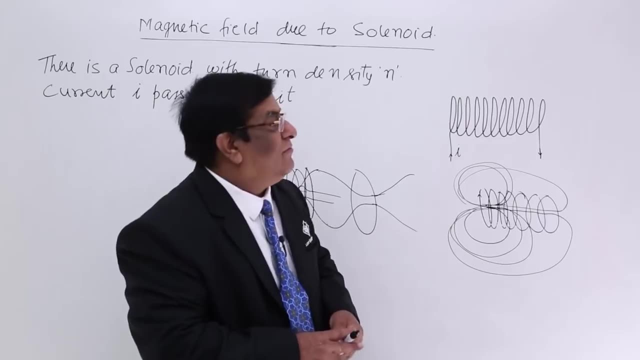 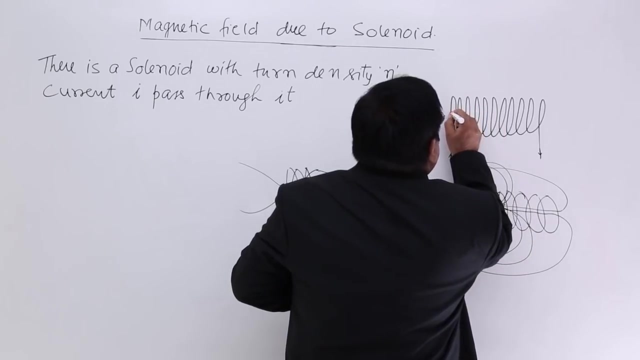 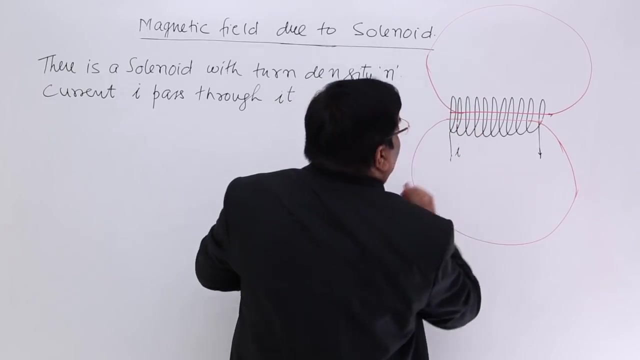 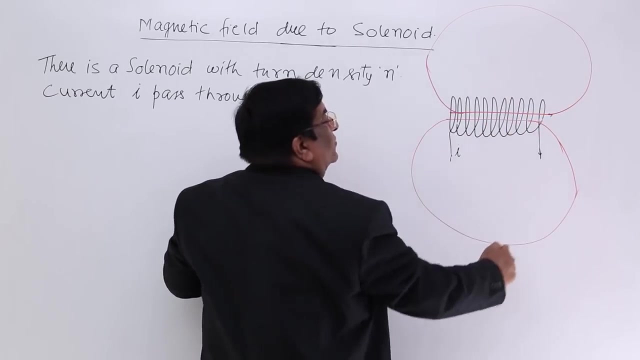 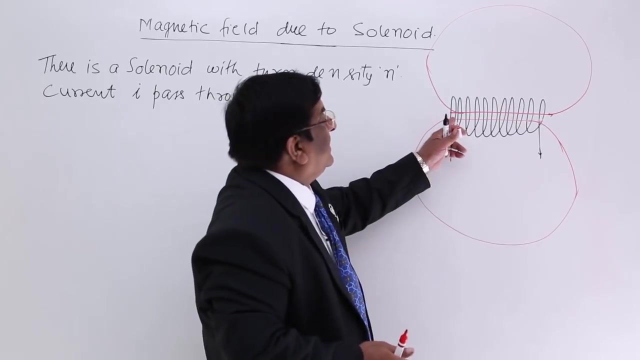 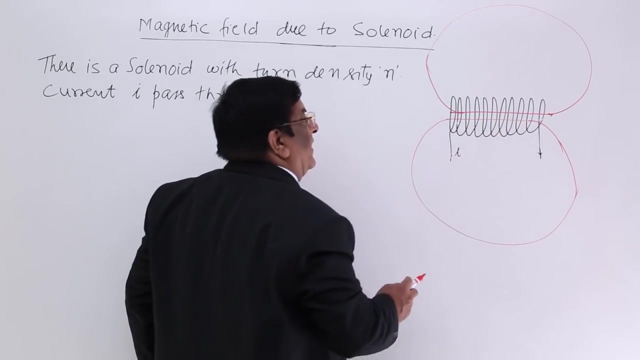 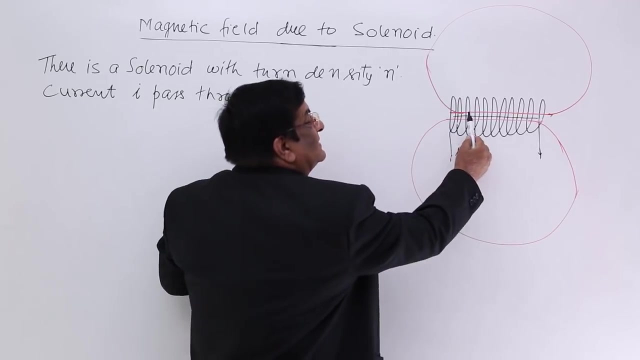 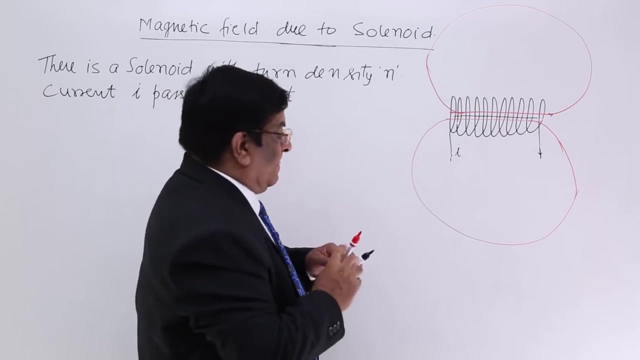 Due to the second term. So inside magnetic field becomes straight altogether from first to the last. This is how magnetic field has a shape inside a solenoid. And when it comes here, then it will go like this. Okay? The current is flowing from the third circle to the fourth circle. So the second turn is like this. So if we bring the current here and then it goes like this. this way this is the magnetic field from the last coil it start turning up it start turning down because it is a closed loop but inside it has no time and it has no space to turn because immediately after one turn there is a second turn very close to it so it has to go straight so inside a solenoid this is along the axis this is axis of the solenoid so this magnetic field is along the axis inside a solenoid outside it spreads out ok. 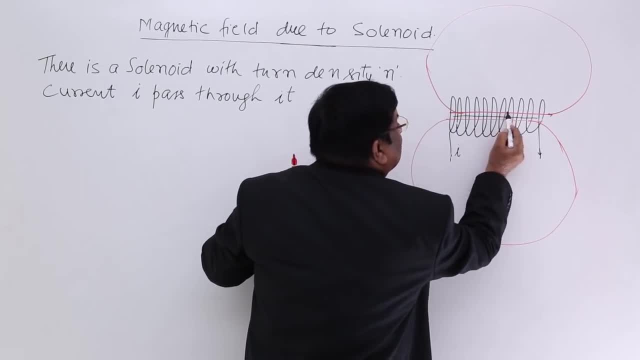 Now if there is a magnetic field here all these magnetic fields are in the same direction 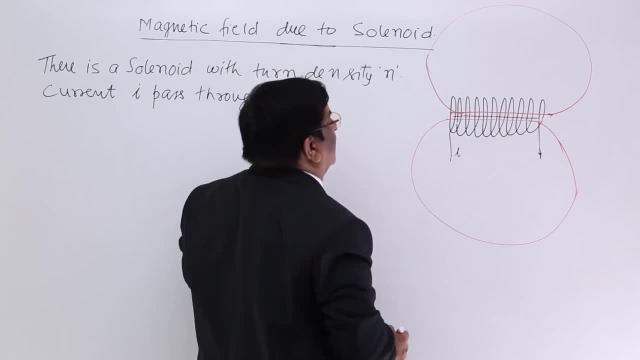 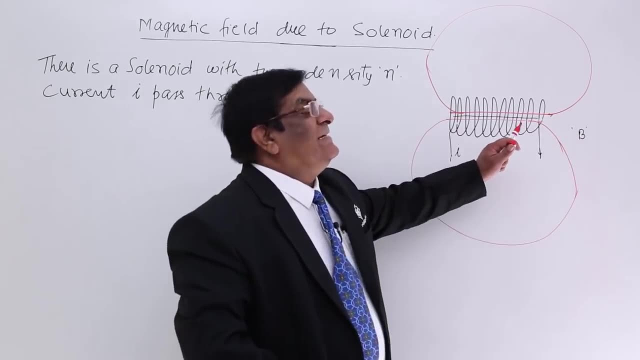 same magnitude so this is a uniform magnetic field let us suppose this has a strength b now we want to find out how much will be this strength b. If 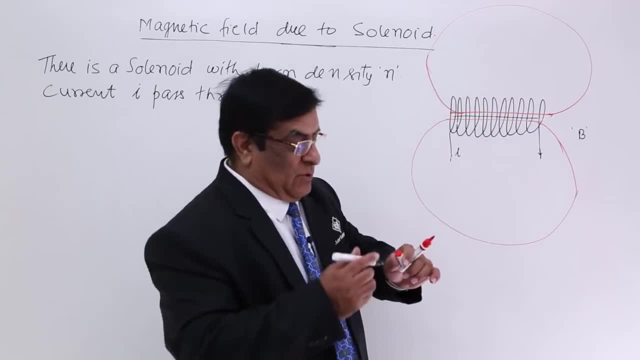 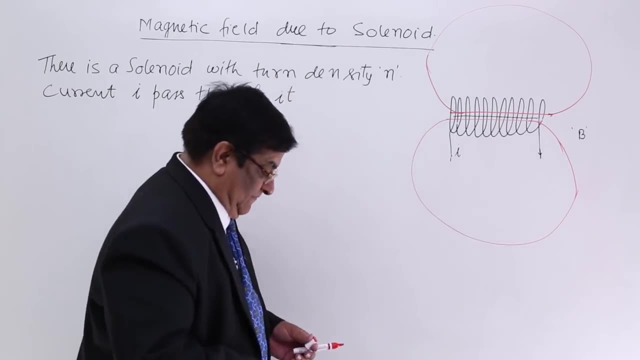 it has a certain parameter ok now we will find out with help of Ampere's law which are the quantities which are affecting it. 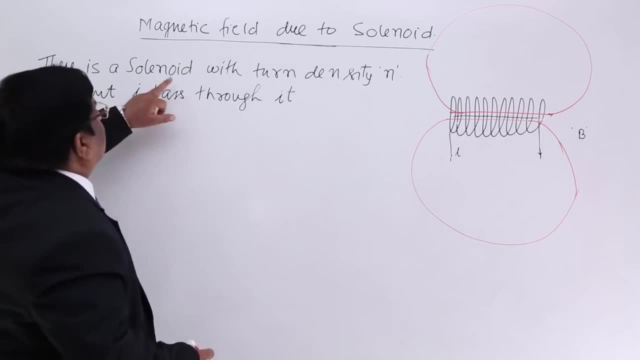 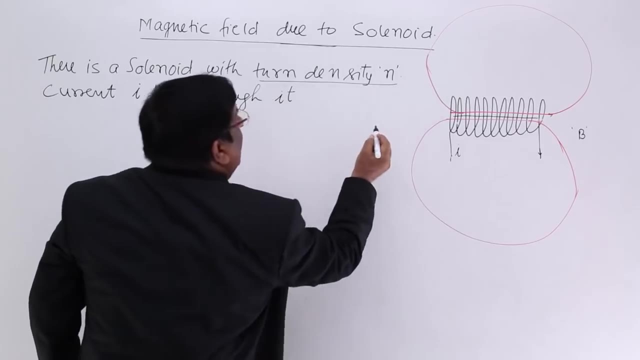 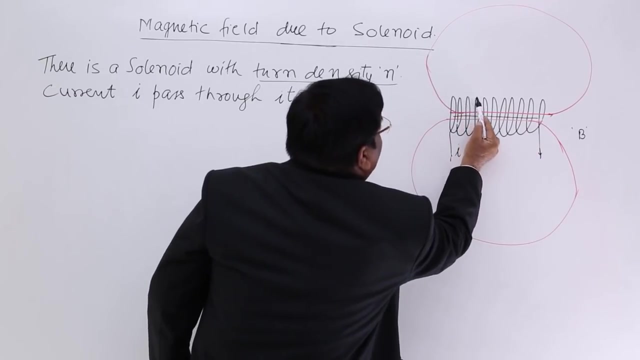 The first thing is there is a solenoid with turn density n what is meant by turn density turn density is in 1 meter there are n turns this 1 meter length has 1, 2, 3, 4, 5, 6, 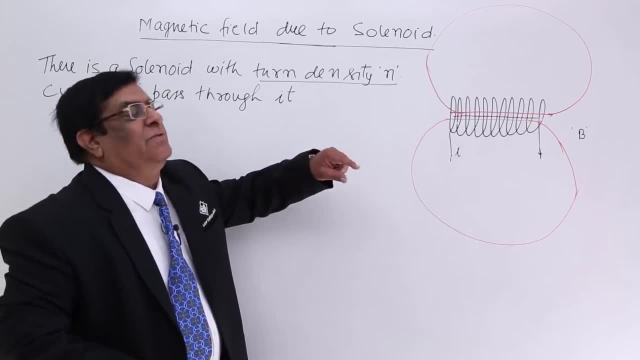 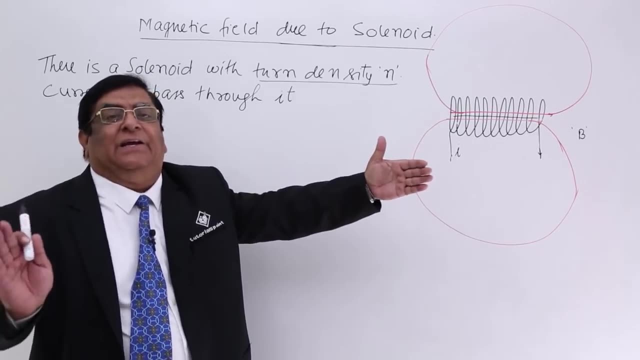 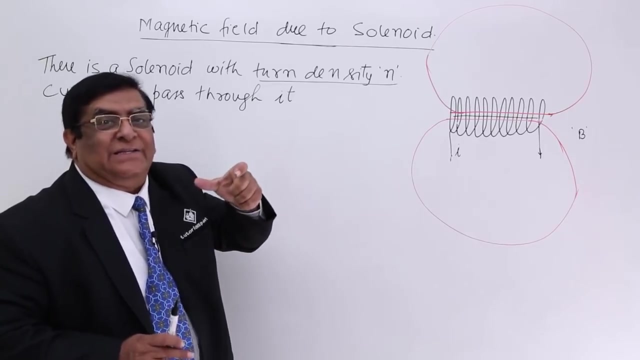 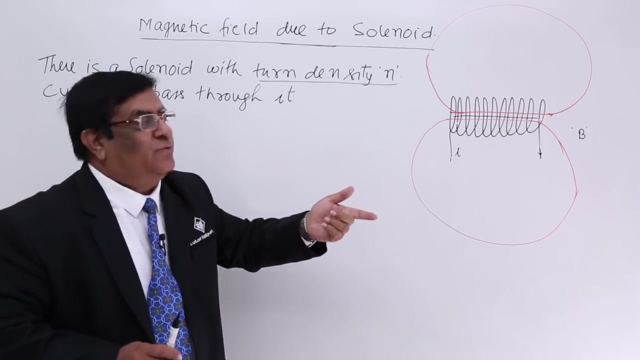 and turns if it has got 300 turns we will say turn density is 300 if it is 2 meter long then the total will be 600 if it is half meter then it will be only 150 because it is 300 per meter so that 300 is n one solenoid can have 300 another can have 100 one can have 1000 so we use a general term n. So, remember. n is. 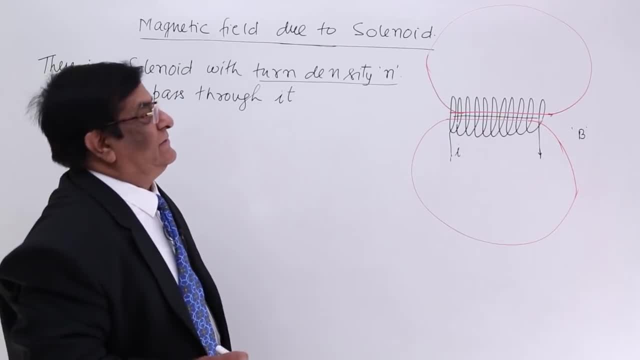 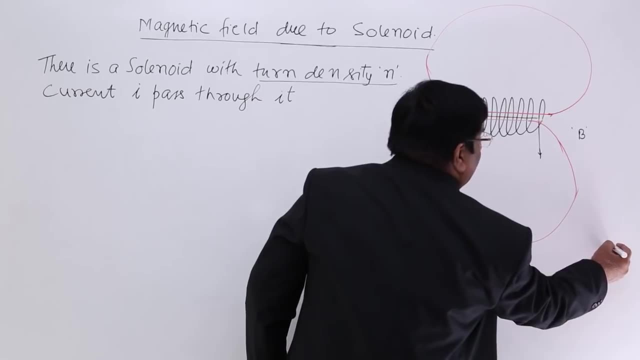 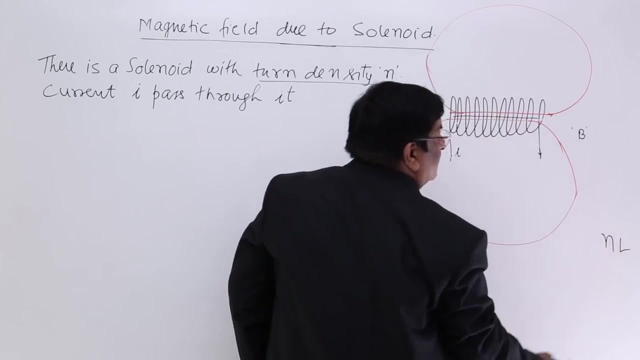 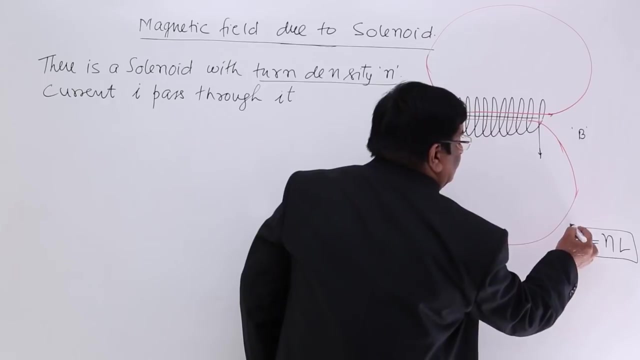 The total number of turns per unit length not the total turns if there is a length equal to L the total length is L if we multiply this L with number of turns per unit length then this will give the total number of turns and we will write it this. This is total number of turns. . length is only L, then multiply with this and this gives the total number of turns. 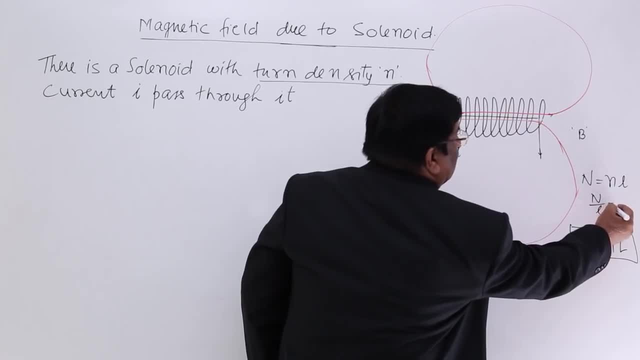 So there is a relation like this, N upon length is equal to N or N into L is equal to this 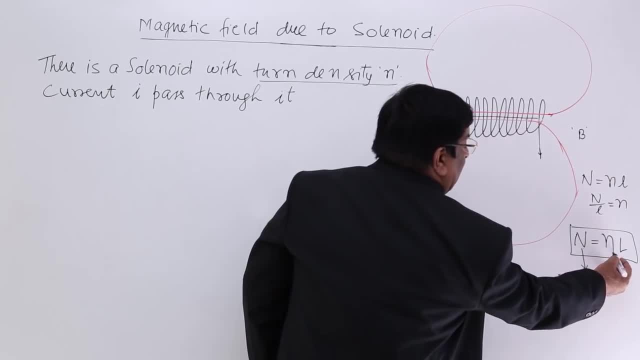 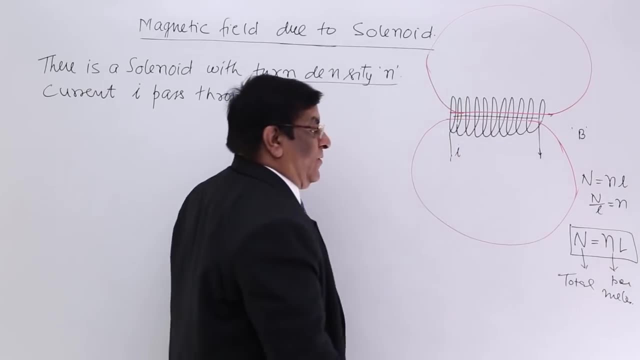 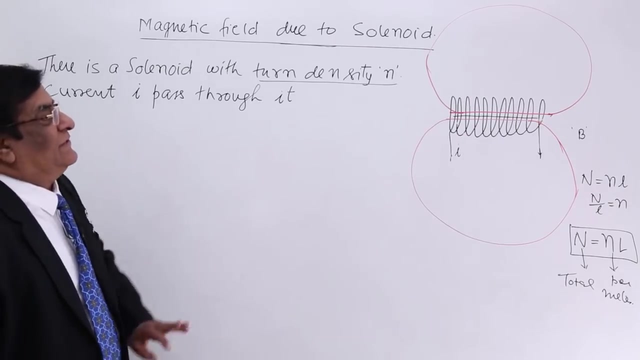 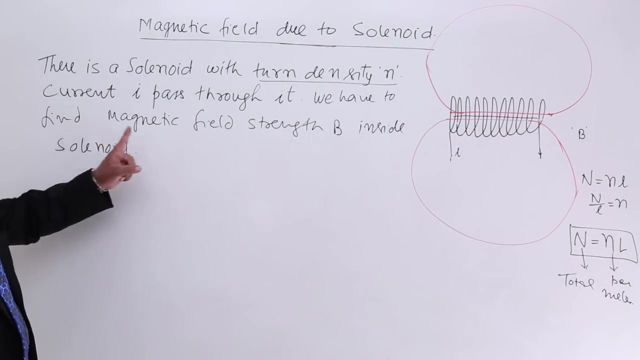 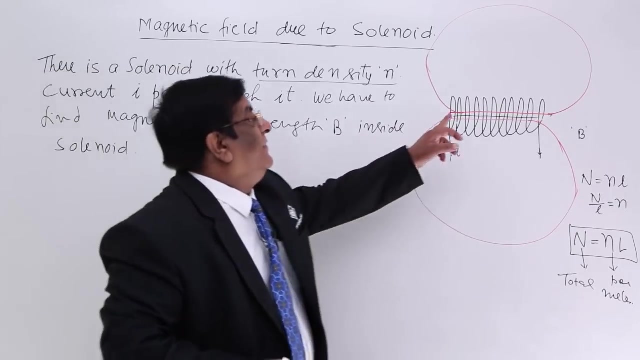 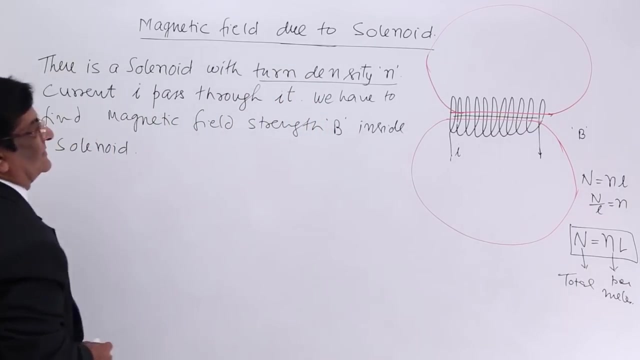 and this is what? Total and this is per meter. So now you understand what is the meaning of N. Current I is passing through this and we have to find magnetic field. We have to find magnetic field strength B inside solidite. Anywhere here we have to find the magnetic field. So we start with Ampere's law. What was our first? Consider an Amperian loop. 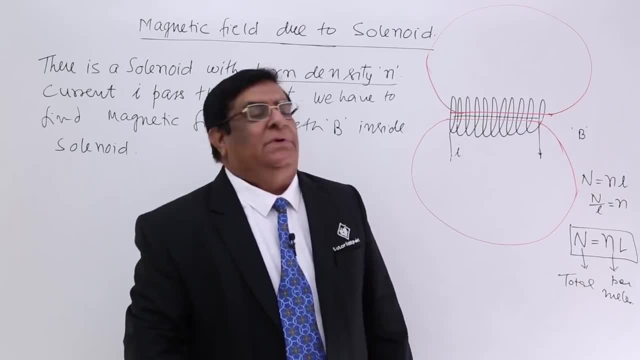 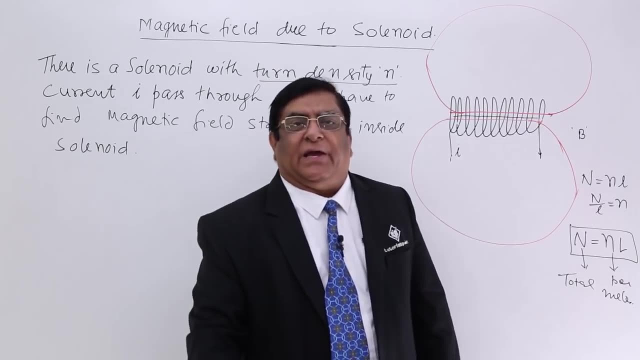 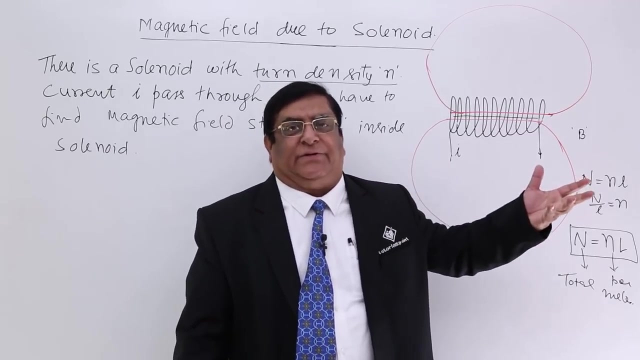 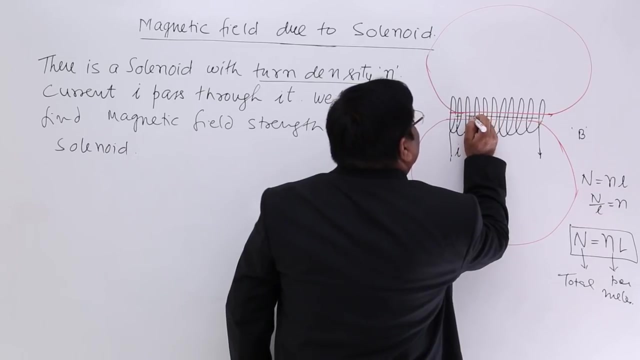 In this case we consider an Amperian loop. But we do not find any Amperian loop which is totally symmetrical. So we have to make an arrangement that some part of the loop will be symmetry and some part will have other type of symmetry. So we make an Amperian loop here and that Amperian loop we take as a rectangle. This rectangle. Okay. This rectangle. Okay. This rectangle. 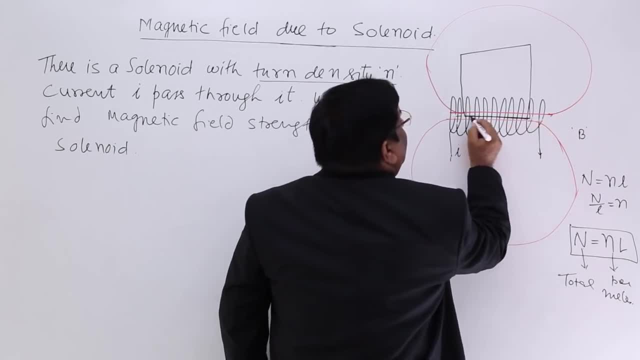 They have seen this is a full length. These two here see. This and this is not full length, it is a small length here. And it goes like this, this, this. This is a rectangle. Okay. 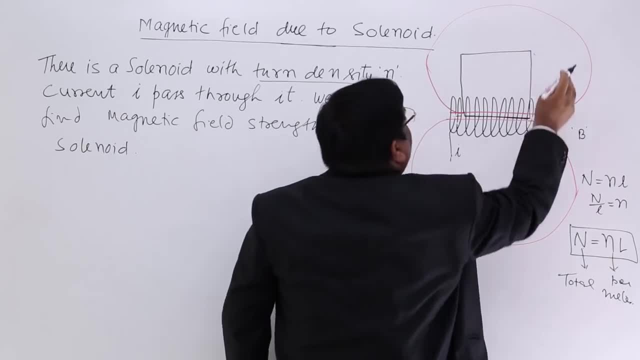 Let us give it a name P, Q, R, S. P, Q, R and here it is S. Okay, this length. salt to simple, so far. 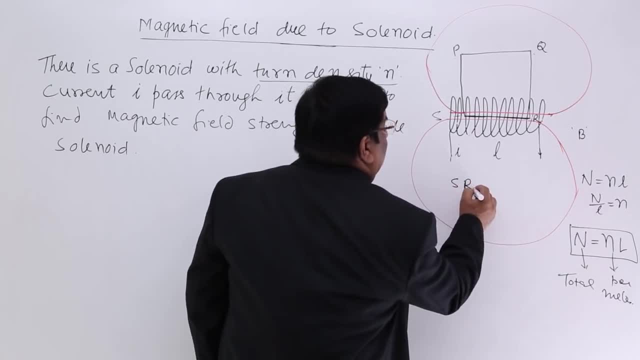 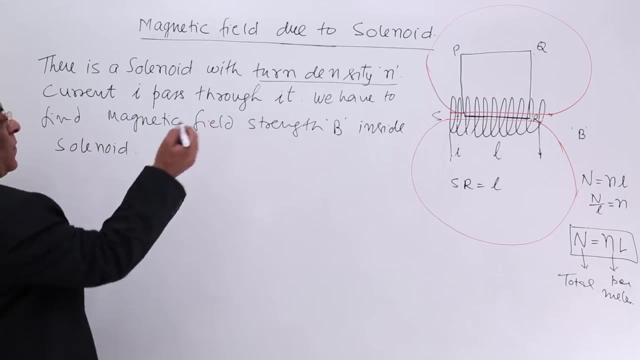 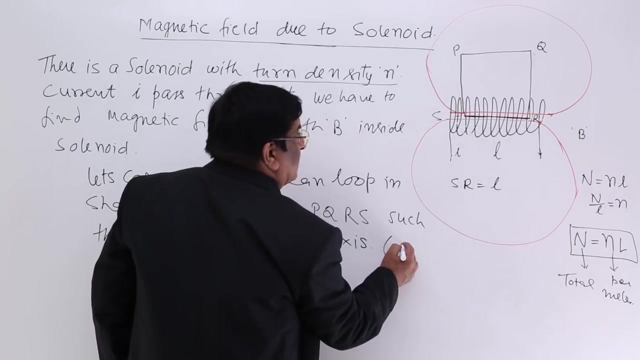 Let this length be small. L. S R is equal to L. This is our loop. One side of this loop in this case S R is along 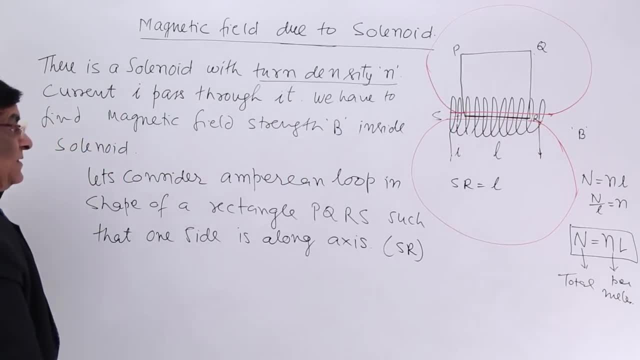 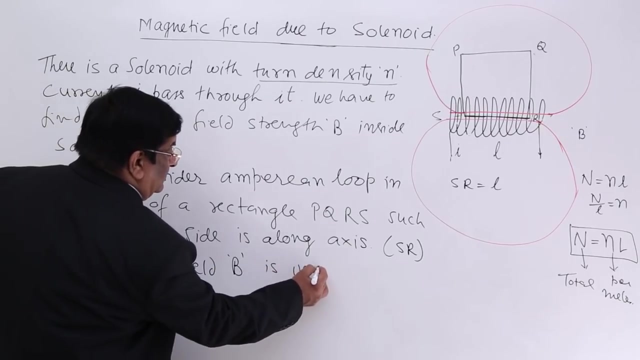 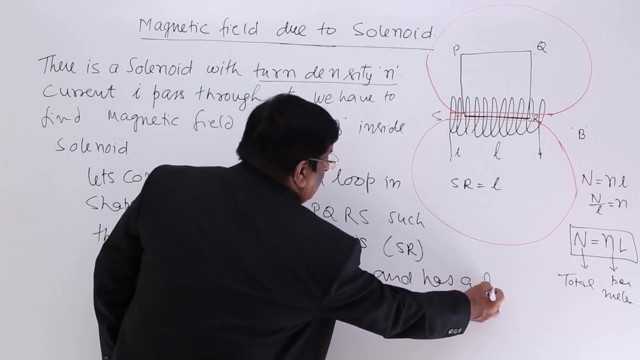 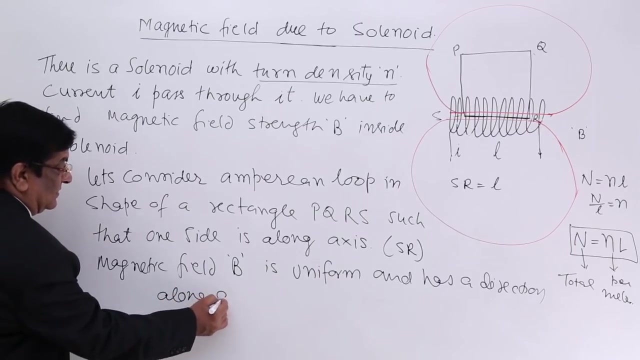 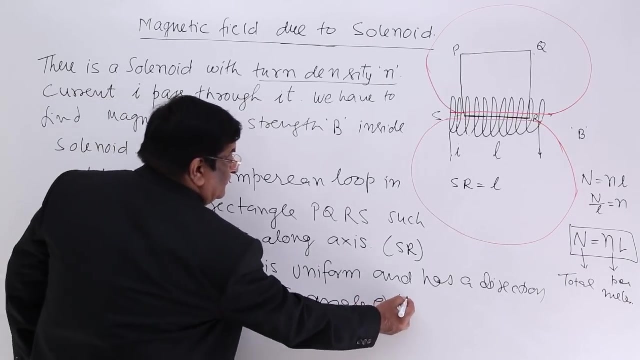 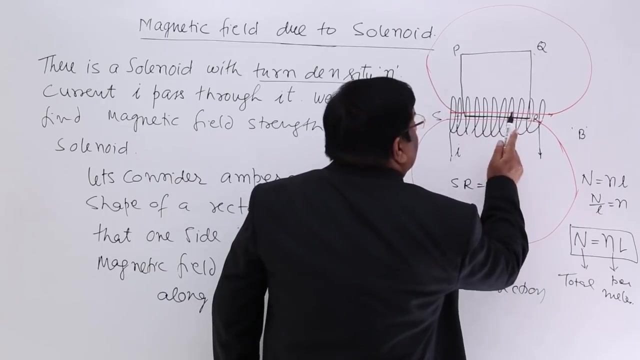 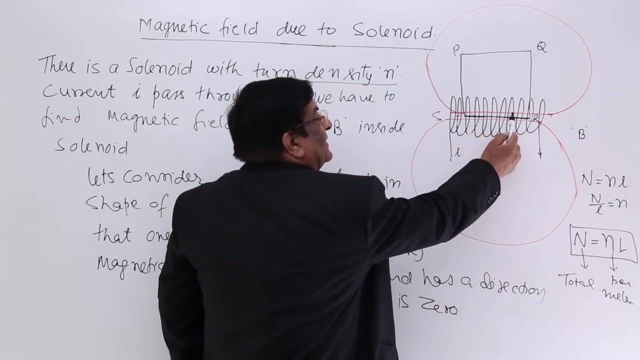 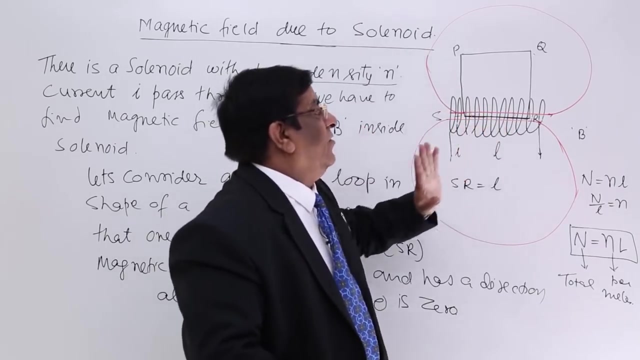 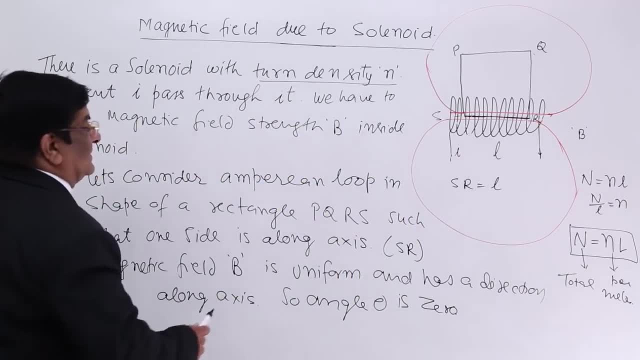 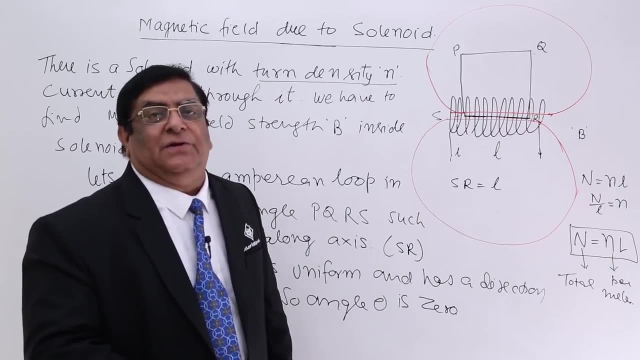 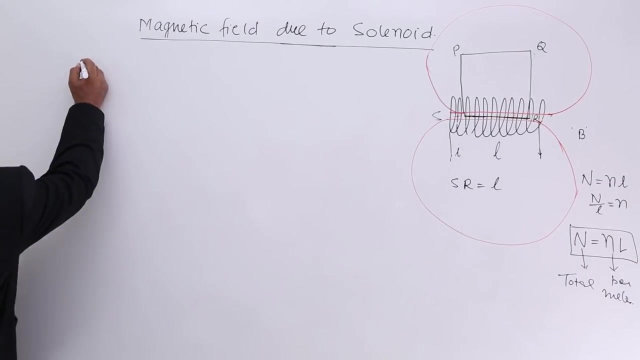 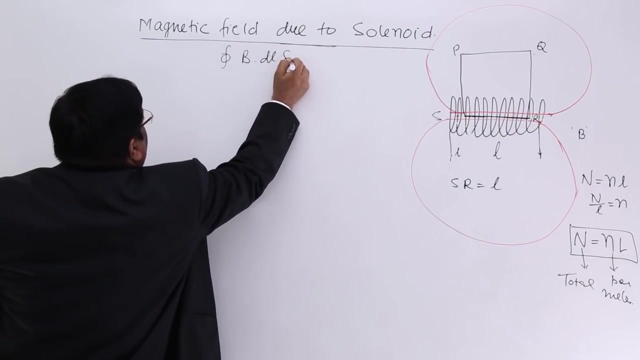 Okay, let it be. So this is our first part. Now we go for the second part and in second part we will start calculation of closed integral BDL. So closed integral BDL we will calculate. Now second part, we know Ampere's equation BDL cos theta. 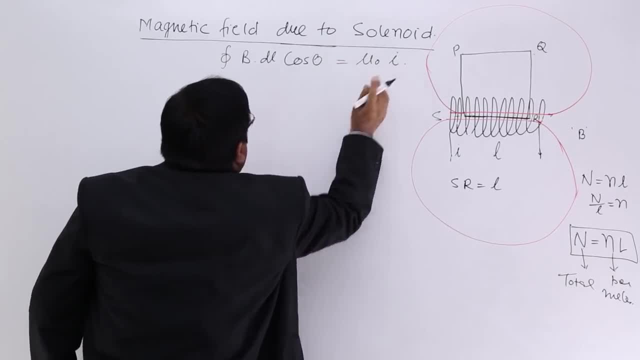 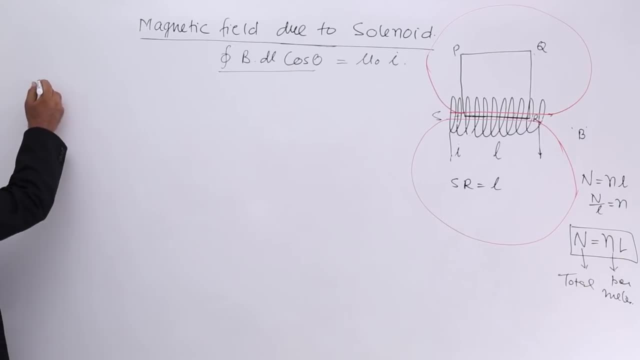 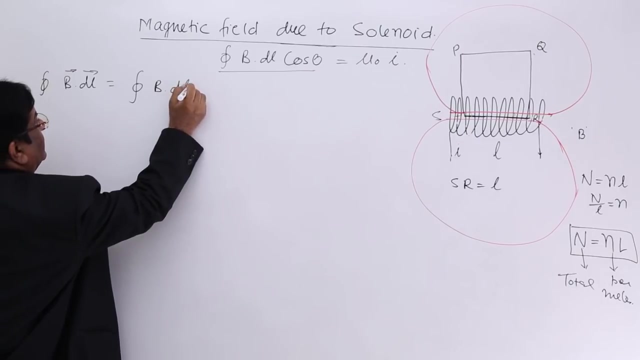 So in the second part, we will do this calculation. With in the second part, we will do this calculation tv comcause 30 sport Now let us draw. That is closed integral BDL is equal to closed integral BDL cos theta. And in the third part, we know that for the whole loop as b is it. So begins to click and the third part we will do this calculation that is for the whole loop. And this is for the complete loop crewsいますok in the consecutive part, we will do this calculation. That is closed integral BDL is equal to BDL cos theta, and this is for the complete loop. Thank you Jetan,an tsou aide. Satna Duck DasDeshenfest and Satna Buttern. The second part we will do is we will do this calculation. 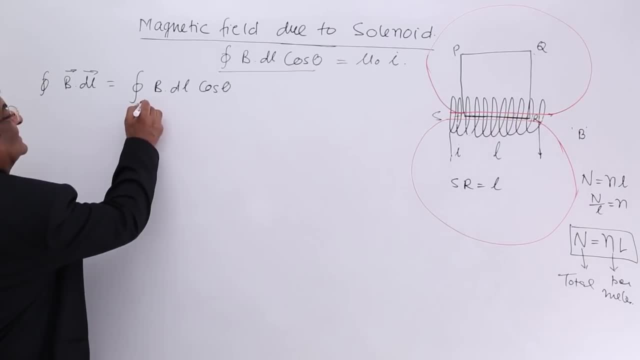 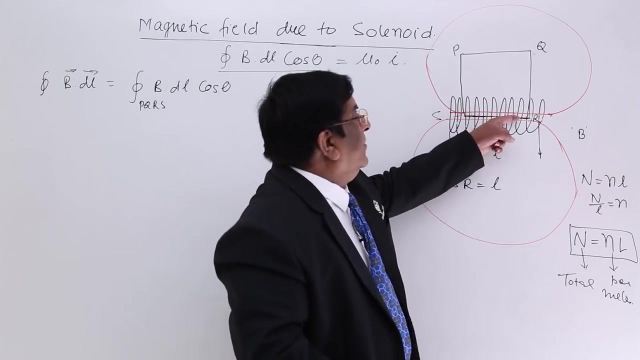 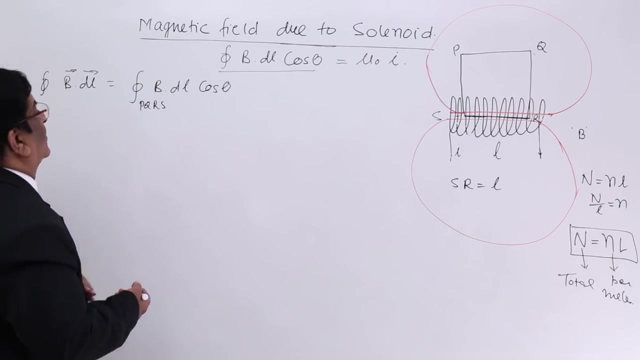 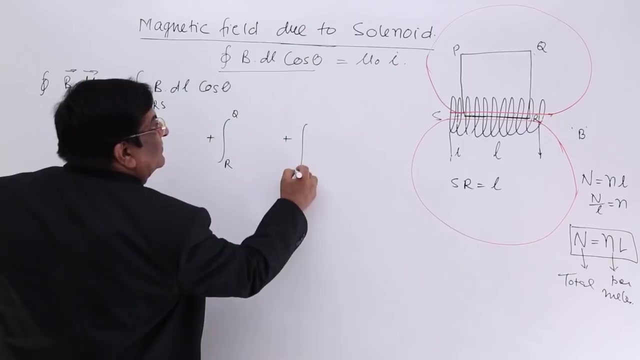 complete loop and what is that loop PQRS. Now, this calculation for integration of DL theta is the angle between B and DL, but here it is 0, but for this part it is 90 degree, for this part it is 90 degree, for this part it is 180 degree. So, what should be the value of theta here? Answer, there cannot be any one value. So, what do I do? I do this calculation in four parts and this I write as this integration for the closed, I will convert it, integration I will do from S to R, then I will do an integration from R to Q, then I will do integration from Q to P and then integration from DL to DL to P. 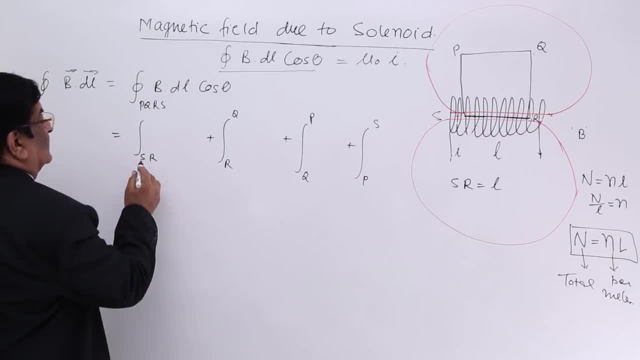 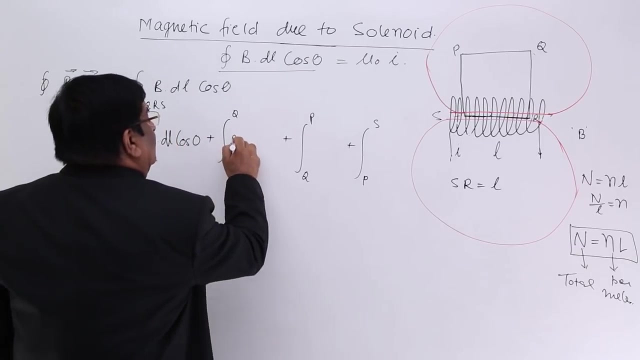 Now, P to S, this S to R is B DL cos 0, because here it is 0. Then for Q R, this is B DL cos 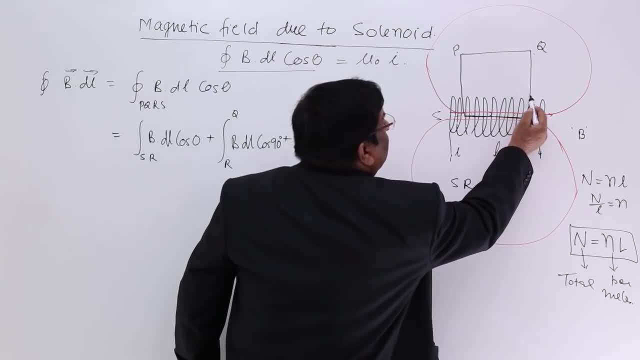 90, because this line and this magnetic field, this are making right. . 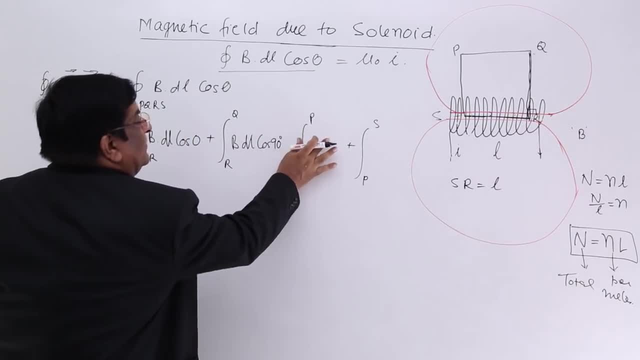 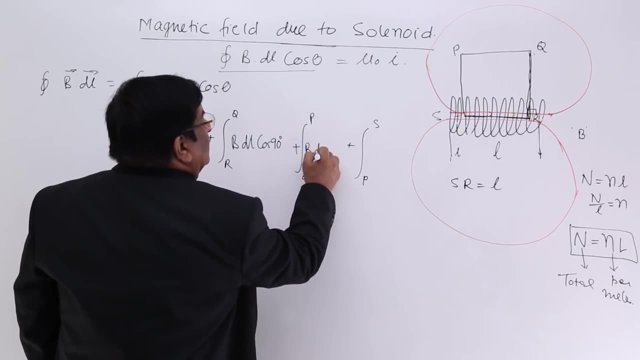 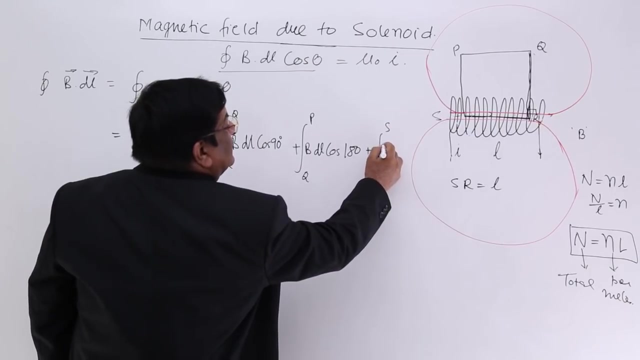 So, this is cos 90 plus P to Q, P to Q is B DL cos 180 and again P to S, P to S, this is B DL cos 90. 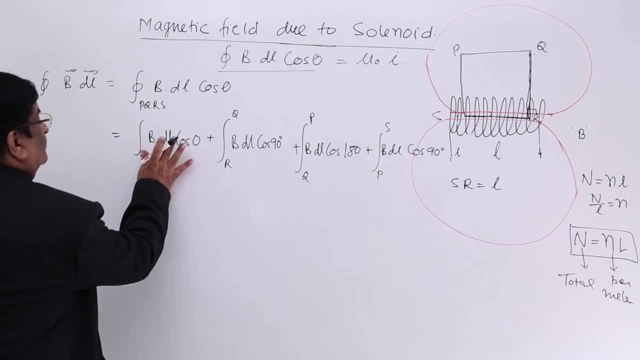 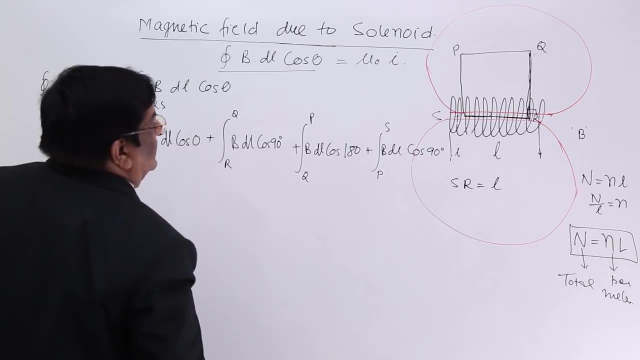 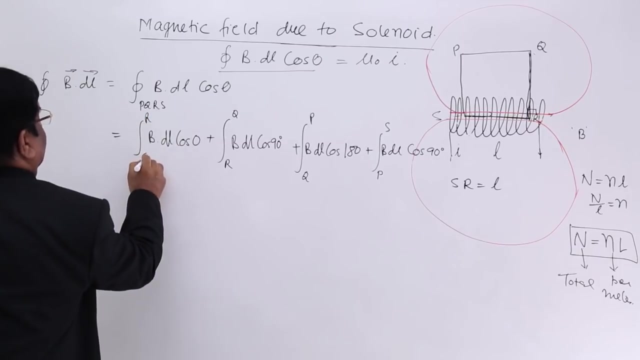 This is I have divided, okay, S to P, P to Q, Q to R and then this is R S, right, S R, R Q, Q P, P S. So, this is closed from S to S, the complete calculation in four parts. 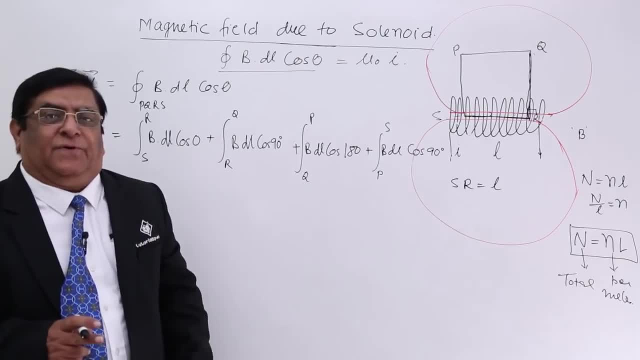 So, this will be our technique. If we do not find symmetry at all the parts of the loop or a surface, we 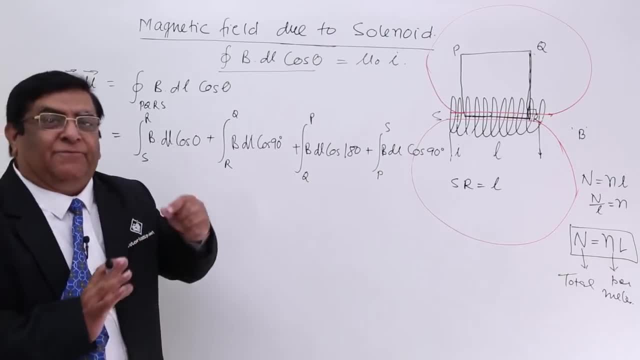 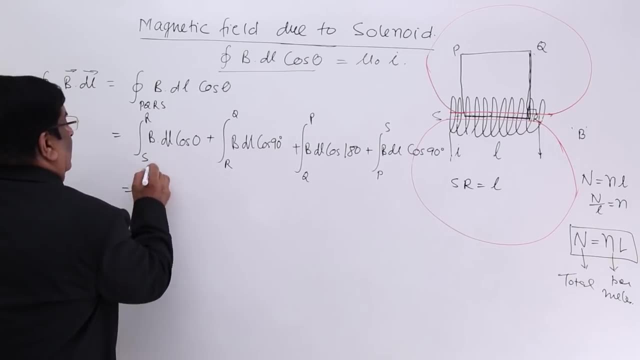 divide it into different loops, so that every individual loop has a symmetry. Here, this whole loop has a symmetry of cos 0. Now, B at every point is same and B, we will have integration of DL. 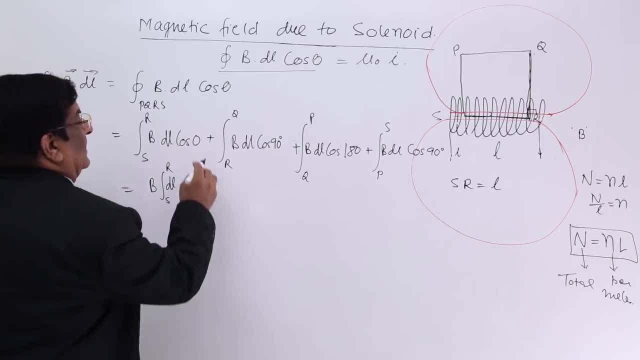 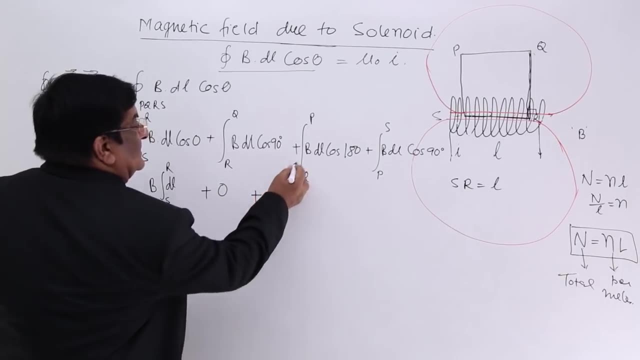 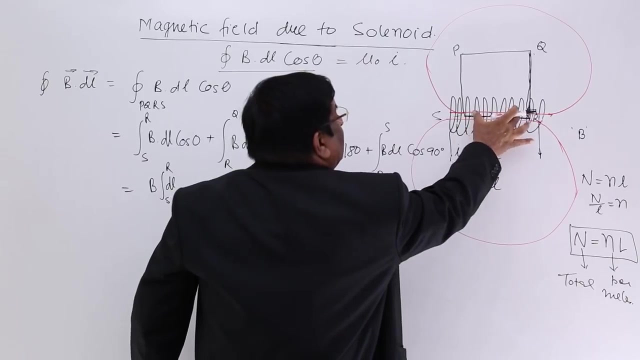 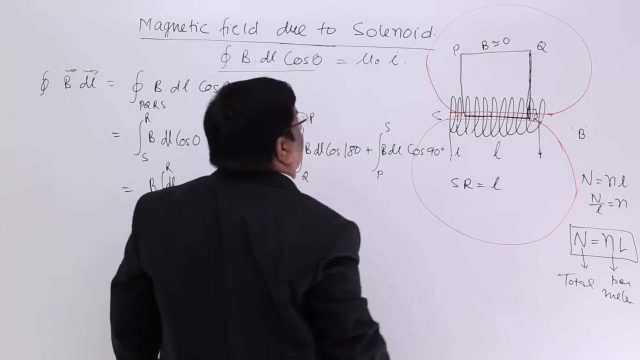 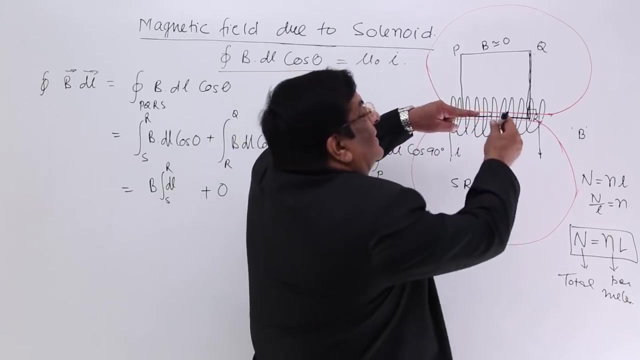 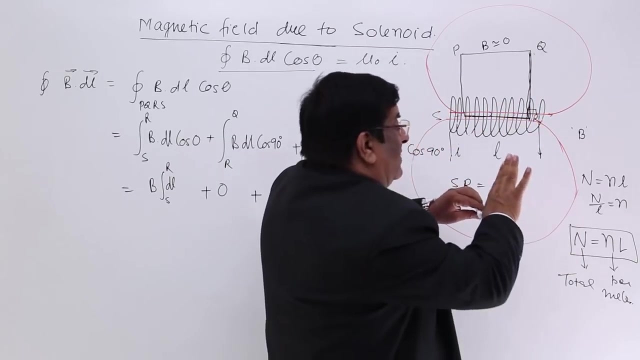 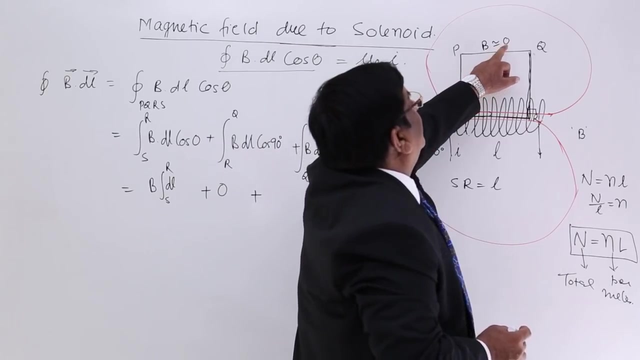 From where to where? S to R, okay. Then, this is plus cos 90 is 0, the whole thing becomes 0. Now, this plus Q to P, this portion. This portion is quite away from the solenoid and we can prove that at P Q, B is almost 0. Why? Here, you see the direction of turn are like this. So, this direction of turn are, this will make a magnetic field in this direction and this one, the one make magnetic field and this one is 0. Then, this one, this one, this one is the straight way. Now, you can see, that if you solve for the magnetic field, it will not be horizontal. If we do the least drooping of the ends of the bank, then the second is neither point, still extend. Into what direction is the current passing? From this one, the mano group of the matrix we get plus or minus 2 to y. It is such that there is no electric feedback at all on the ambience. Now, besides that, there is no other magnetic available and this one is not. Now if we converge these two expansion from negative to positive, then we'll get the previous holistic factor of field restaurants. 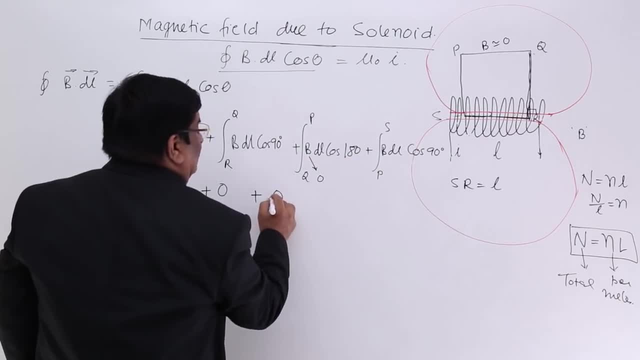 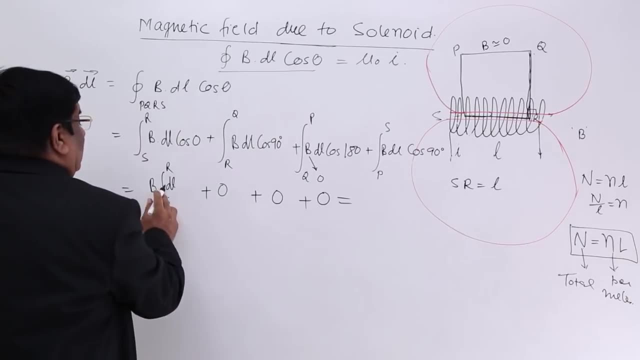 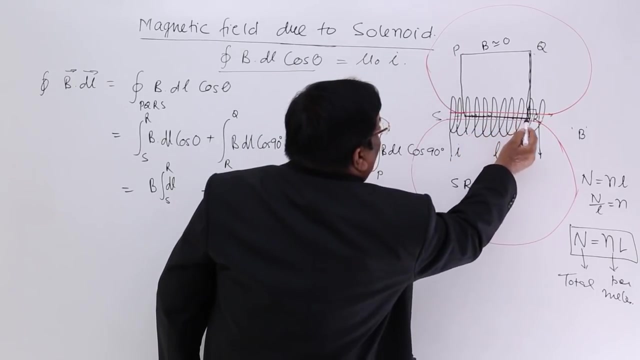 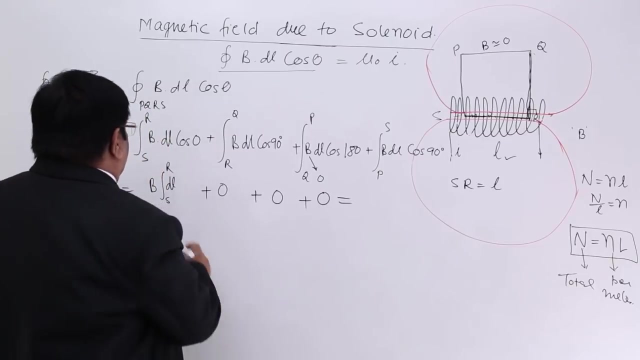 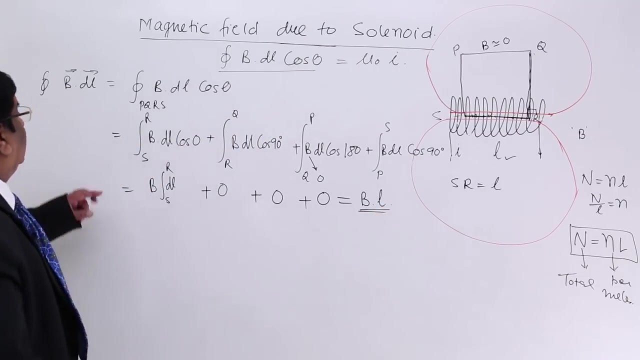 become 0, so this whole thing become 0. Then again cos 90 is equal to 0, so this is 0. Now we get this B integral dL from S to R. From S to R if we add up all the dL, what will be the addition or the integration of all the dLs that will be equal to L. So this we can write as B into L, B into L. This is closed integral B dL for the entire Empyrean loop. Now next part, third calculation we will do. 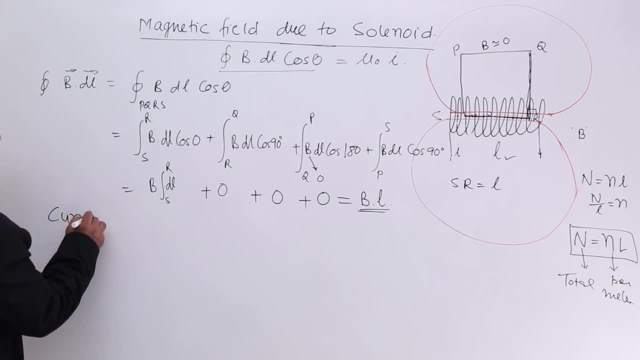 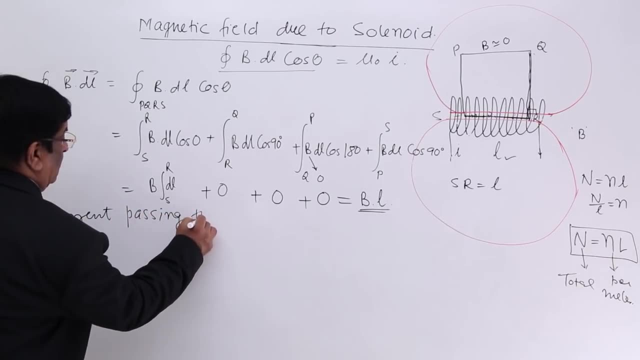 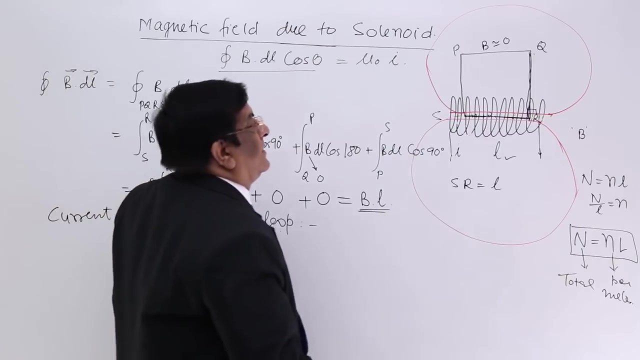 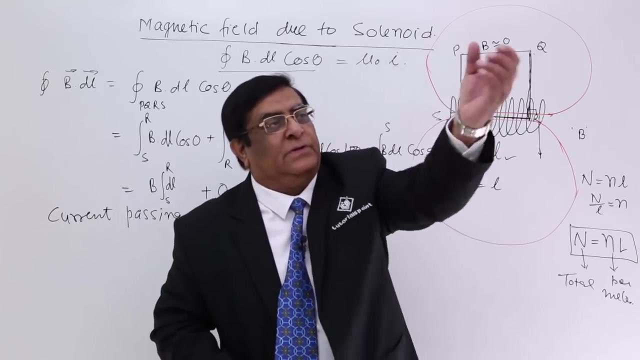 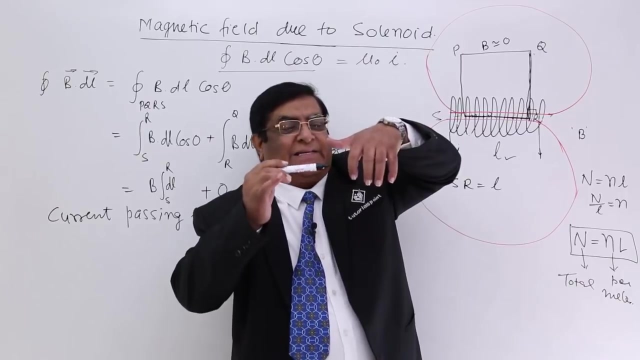 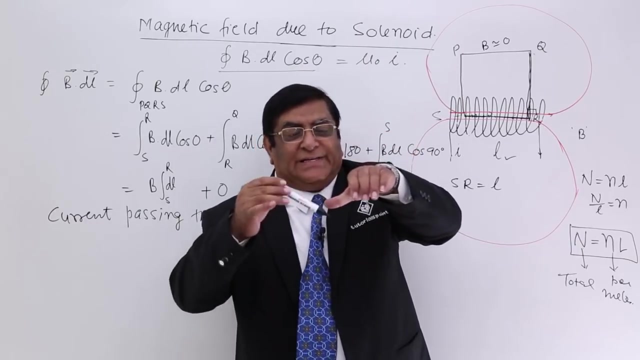 What is the current passing through the loop? And this is to be understood well. Current passing through loop. Here in one turn current is I. How is the loop? See this is solenoid turn which are like this and the axis is this way. Where is the loop? The loop is here. Now if the current is passing through this. 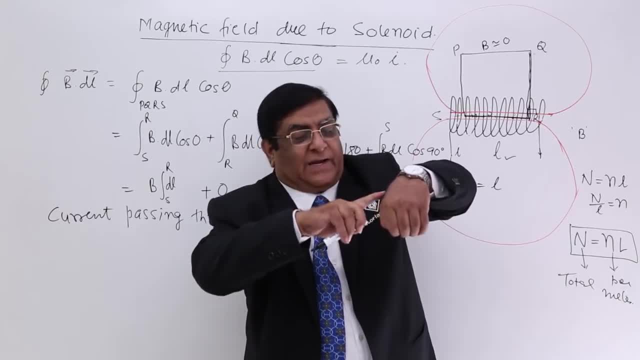 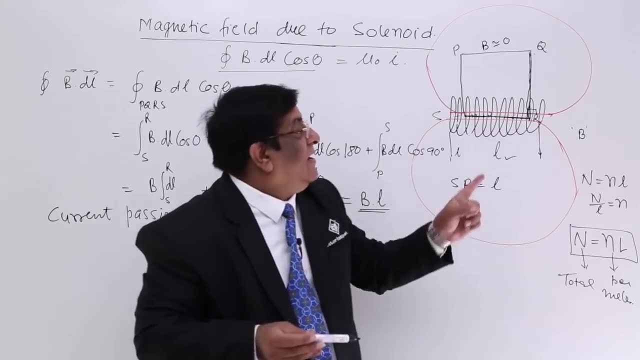 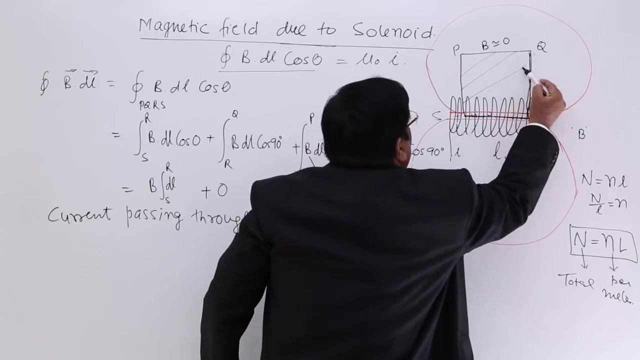 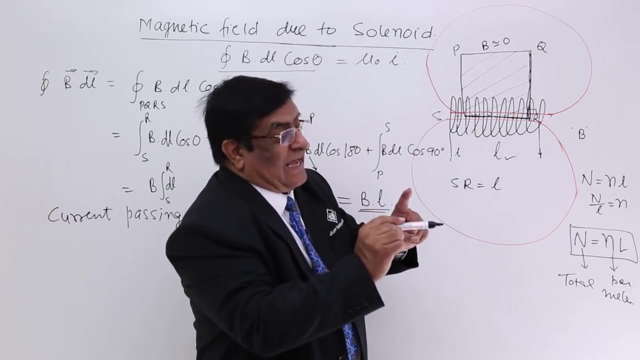 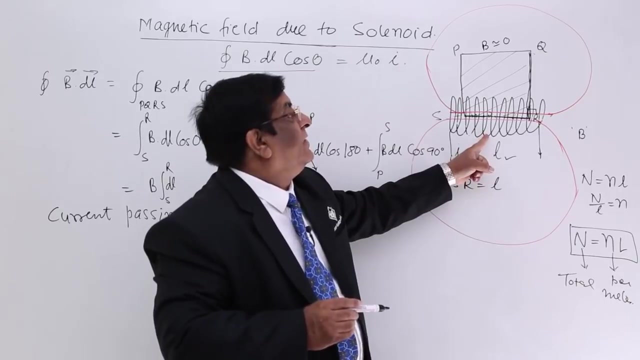 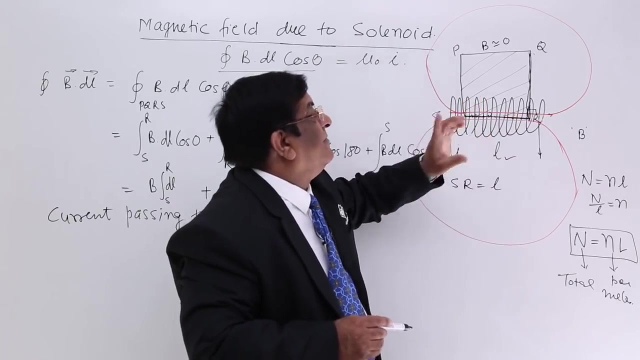 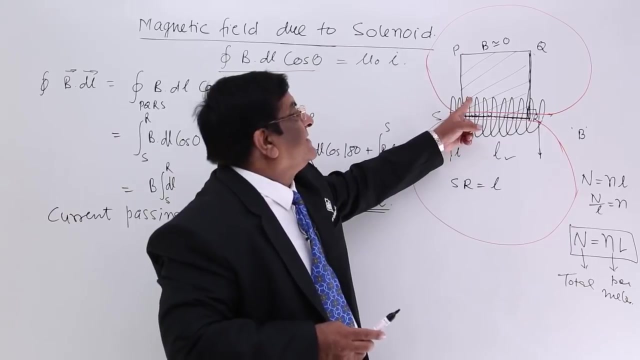 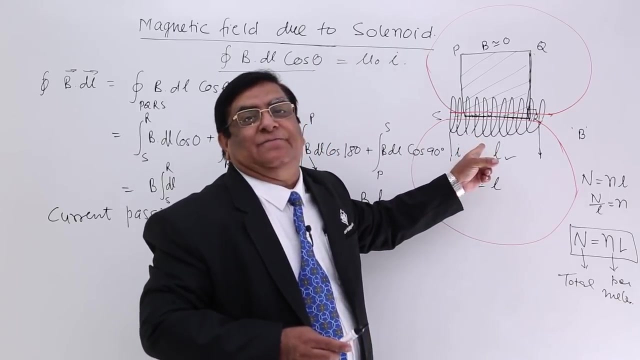 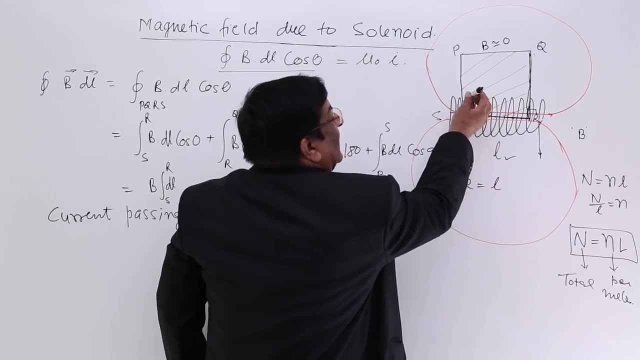 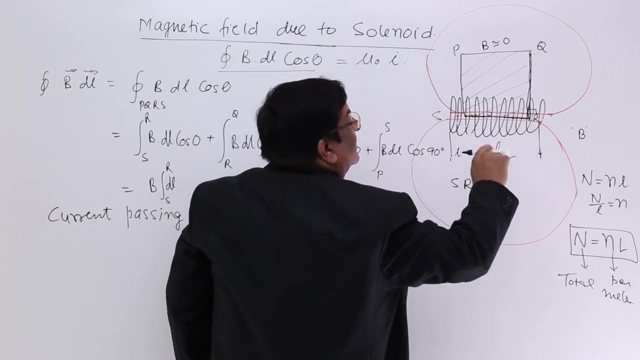 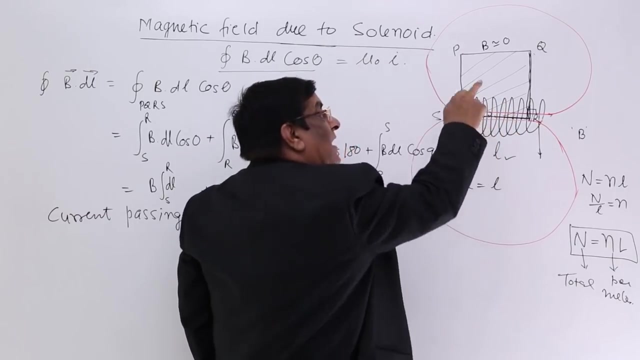 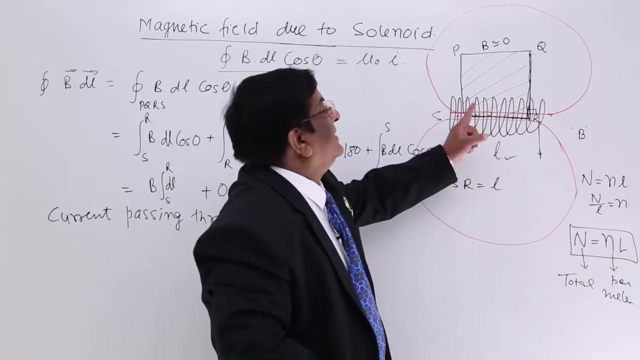 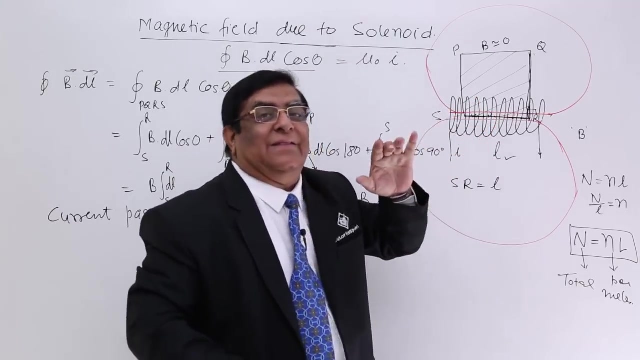 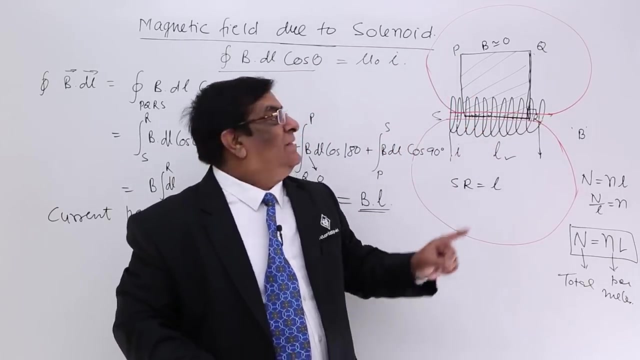 And the loop is this way, then this is the current which is threading through the loop. This current is out of the loop. Where is the loop? This is the loop. You see, this top portion of the circle, this carries the current in the loop. But the bottom portion of the circle is out of the loop so when we say current passing through the loop we should calculate this current this current this current but we cannot calculate this this this or this what is the difference in these two currents number one this current is coming out this is plus i this current is going in this is minus i so this is plus i this is minus i but what we are getting the threading threading is plus i second plus i third plus i fourth plus i is there any minus i answer there is no minus i within the loop minus i is out of the loop so inside there are all plus i if you say these are minus ok inside all are minus then plus are not there that means only in one direction it is coming and this is happening because we have taken our loop very intelligently that our loop will not go up to this point otherwise plus i minus i both will make it 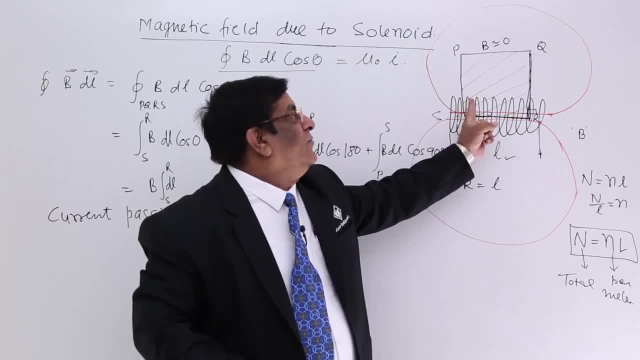 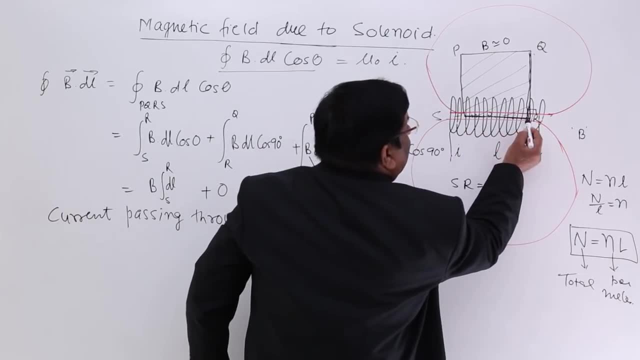 zero here it is only plus i coming out coming out coming out then how many turns are coming out answer is this length is l for every one metre there n turns n turns the length is 15.ены 15.eny 15.eny